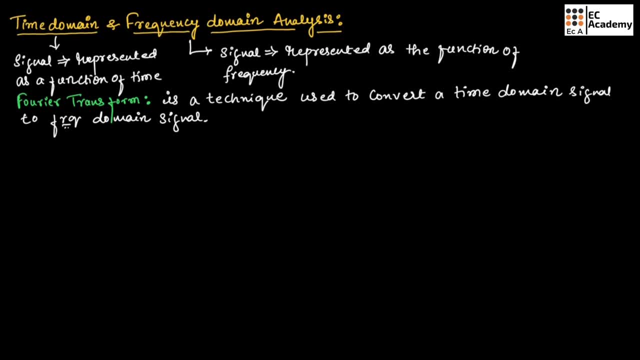 from time domain to frequency domain signal. for example, if we take a signal M of T, for this, if we perform Fourier transform will obtain a signal which will be capital M of F. similarly, if we take a signal S of T, if we perform Fourier transform on that, so we will obtain the signal capital S of F, so M of. 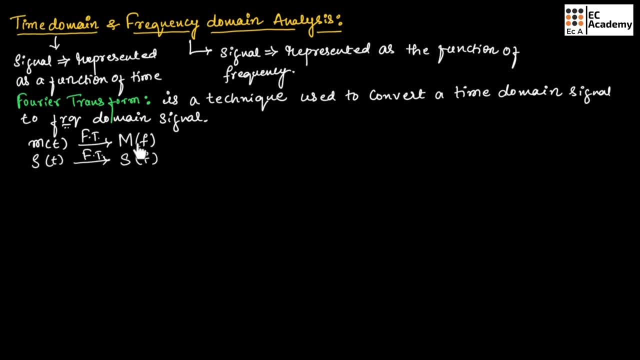 T is the message signal in time domain, M of F is the message signal in frequency domain. in the same way, S of T is the modulated signal in time domain and capital S of F is the modulated signal in frequency domain. if we represent this signal, M of 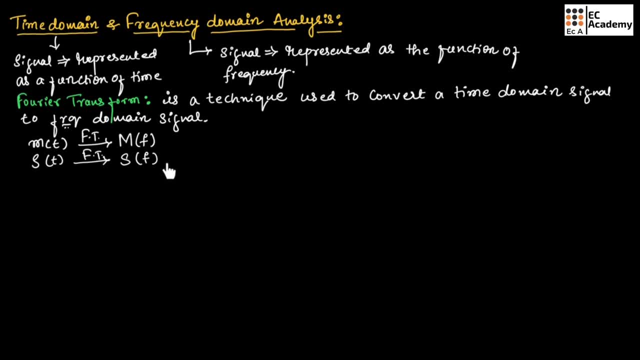 F and S of F. graphically the process is known as a spectrum. so graphical representation of frequency domain signal is known as spectrum. so we can say: the frequency spectrum will give details of frequency components in a signal. so graphical representation of frequency thick mind signal is known as a spectrum and frequency spectrum gives the details of. 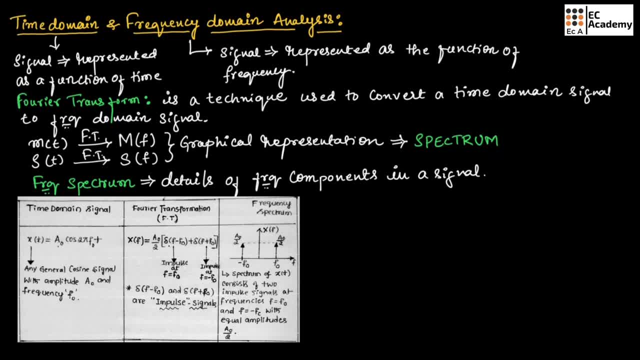 frequency components in a signal. now let us see Fourier transform view standard. back to our standard time domain of còn chicken problem practicing and usingxi signals. Let us take a time domain signal. Then that time domain signals are converted into frequency domain signal using Fourier transform and finally we will write the frequency spectrum. 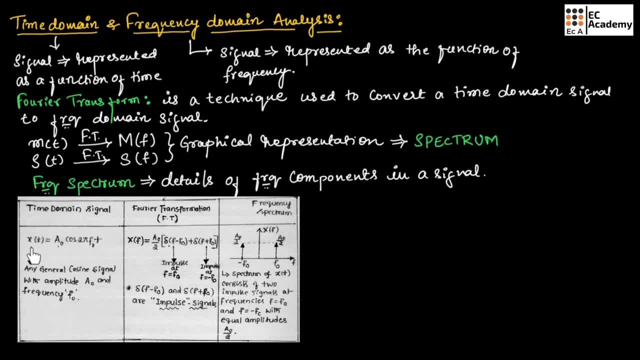 Now let us consider an example of a sinusoidal signal that is represented as: x of t is equal to a naught cos 2 pi f, naught t. This x of t is any general cosine signal or sinusoidal signal with amplitude a naught and frequency f naught For this signal. if we perform Fourier transform, 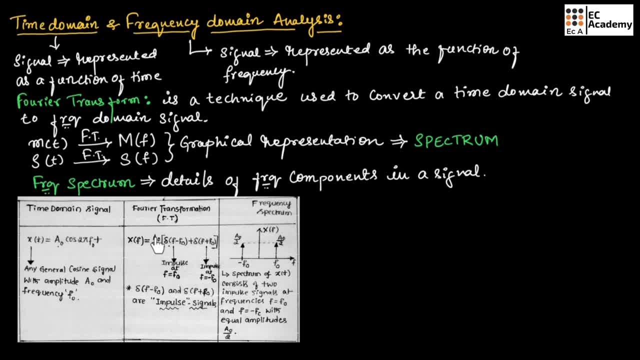 we will obtain: x of f is equal to a naught by 2 delta of f minus f naught plus delta of f plus f naught. So here delta of f minus f naught is equal to a naught cos 2 pi f, naught, t. This x of t is any general cosine signal or sinusoidal. 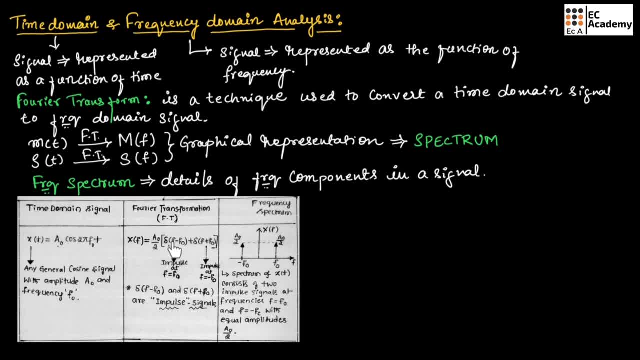 signal. So here delta of f minus f naught is impulse function at frequency f is equal to f naught, and delta of f plus f naught is impulse function at f is equal to minus f naught. So here delta of f minus f naught and delta of f plus f naught are impulse signals. Now this signal is represented. 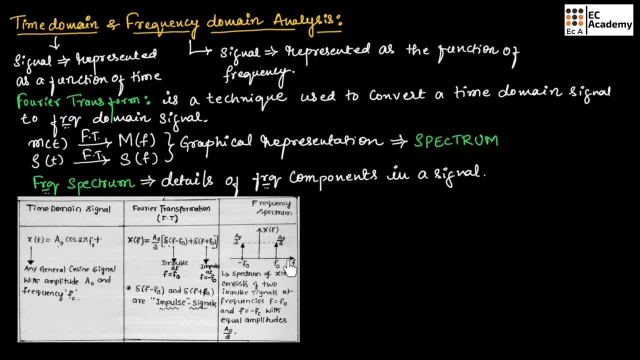 graphically. So here to represent this signal graphically, we will take in x axis the frequency, in y axis the signal which is being represented Now. as you can see, we are having a delta function at frequency f is equal to f naught. So we have written a delta function or impulse function at. 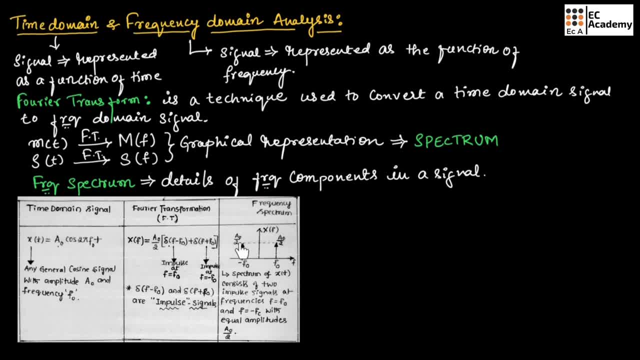 f is equal to f naught. and we have written one more delta function. at frequency f is equal to minus f naught. Both this impulse function will be having the amplitude a naught by 2.. So this is the amplitude. So this is how we can represent the signal graphically. Now let us consider one more signal. 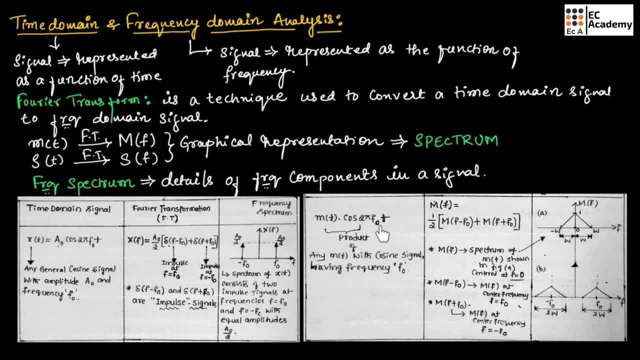 which is m of t into cos 2 pi f naught. This is the product of message signal m of t and sinusoidal signal or cosine signal with frequency f naught. The frequency domain representation of the signal can be given as 1 by 2 m of f minus f naught, plus m of f plus f naught. So 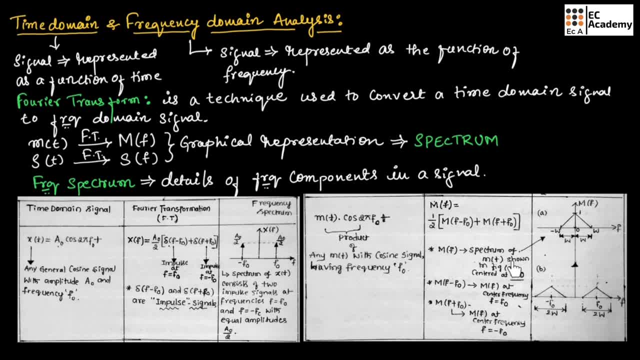 here the m of f is the spectrum of the message signal. So m of f is the spectrum of message signal which is multiplied with sinusoidal signal. and m of f minus f naught is m of f at f is equal to f naught. and m of f plus f naught is m of f at f is equal to minus f naught. So this is the representation of m of f. So to represent m of f plus f naught. so this is the cours utmost. 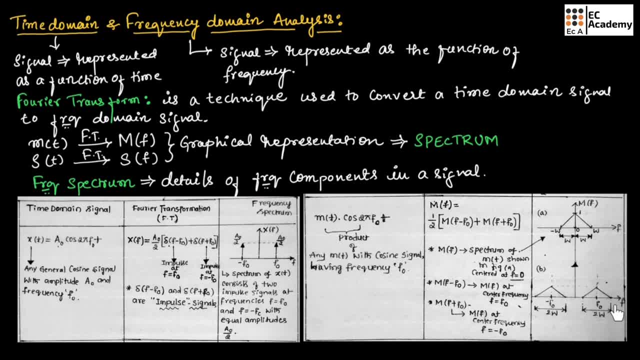 f minus f naught, we need to take the frequency f at f naught and at minus f naught We need to write the same signal: m of f at f is equal to f naught and f is equal to minus f naught.